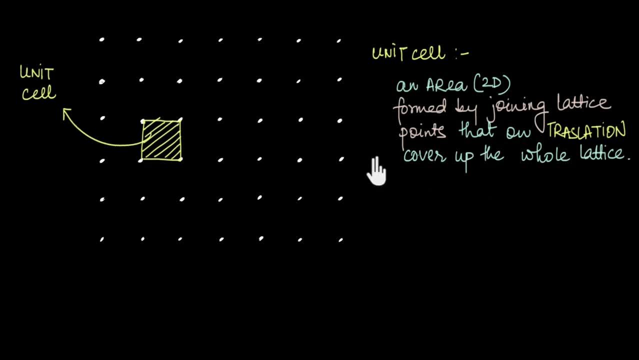 It can cover up the whole lattice Now, because this lattice can be thought to be made up of squares, so we can like go ahead and call this a square lattice. Now, are there other ways of describing this lattice, using some different unit cell? 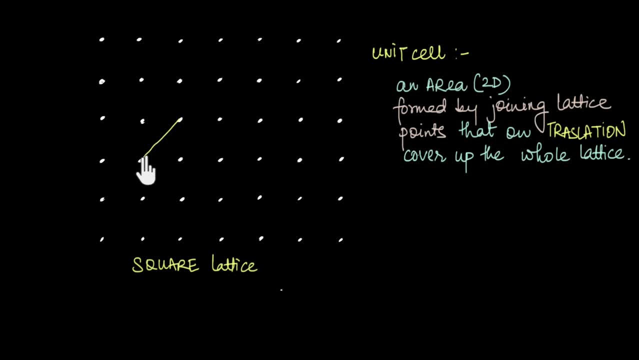 Can we describe this lattice using, say, a triangle as my unit cell? Can a triangle on translation cover up this whole lattice? You can pause the video and think about this for a moment. Well, if we took this triangle and if we translated it? 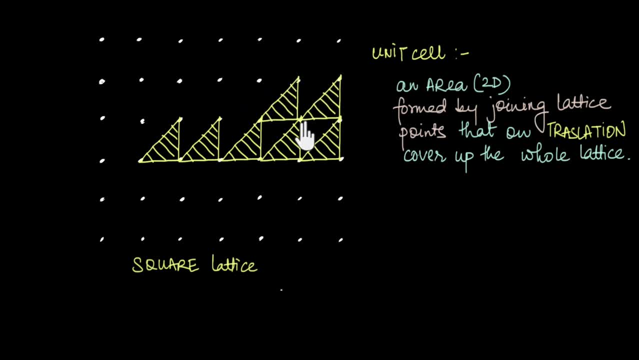 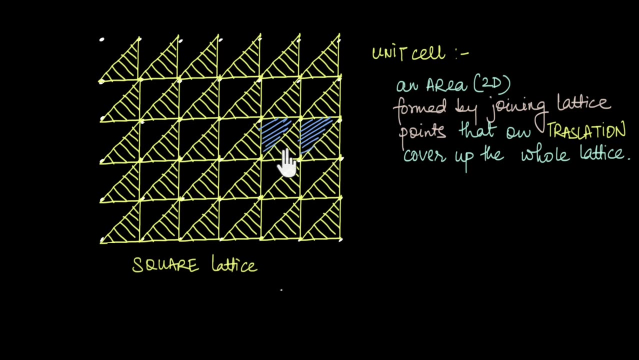 if we did that, we will realize that there will always be these gaps that are left behind Right. so a triangle, on translation, does not cover up a whole two-dimensional space. There will always be these gaps left behind. So a triangle cannot be considered to be a unit cell. 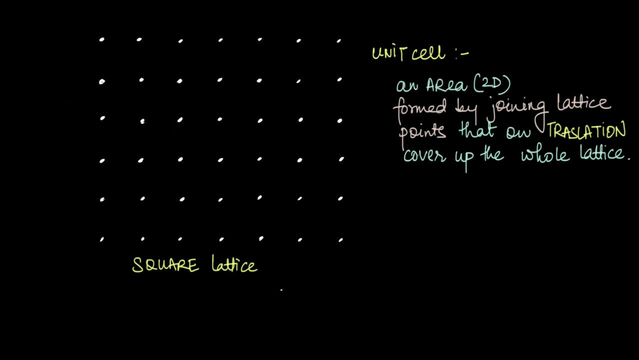 Now that a triangle is out of the picture, what about using this parallelogram as a unit cell? Well, of course we can use it right. If we take this parallelogram and if we translate it, then we can say that the space is just a unit cell. 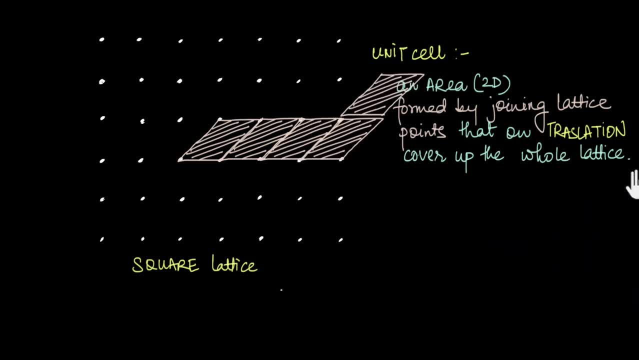 That is right. And because this lattice is infinite in all directions, so this parallelogram can cover up the entire space of the lattice, right? So even this parallelogram can be considered as the unit cell Now, because this lattice can now be thought to be made up of this oblique shaped parallelograms. 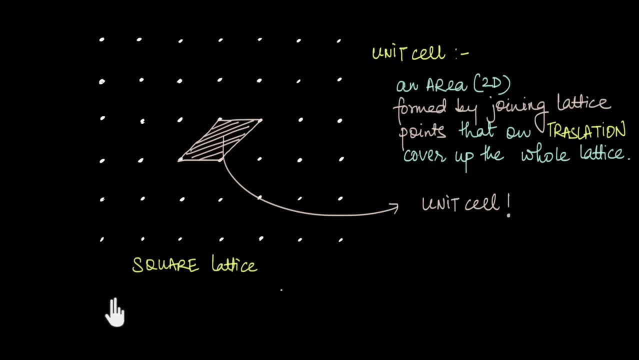 so instead of calling it a square lattice, we might have called it an oblique lattice instead. right Now, besides this parallelogram and the square, there are also many other ways of selecting a unit cell. We can, for example, take this rectangle made by joining all these lattice points. 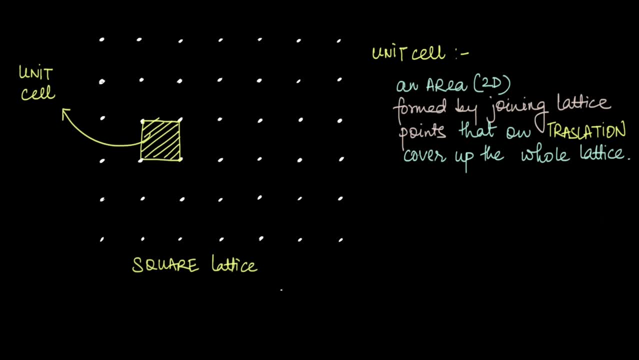 Now, are there other ways of describing this lattice using some different unit cell? Can we describe this lattice using, say, a triangle as my unit cell? Can a triangle on translation cover up this whole lattice? You can pause the video and think about this for a moment. 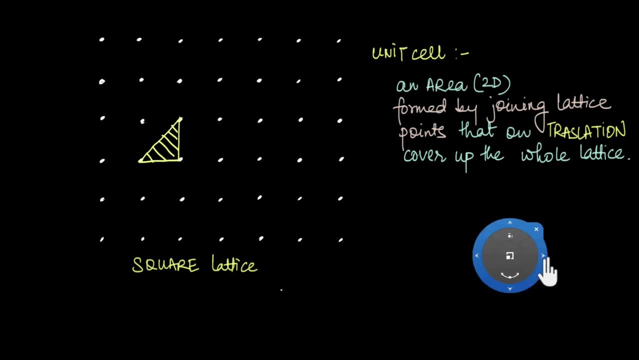 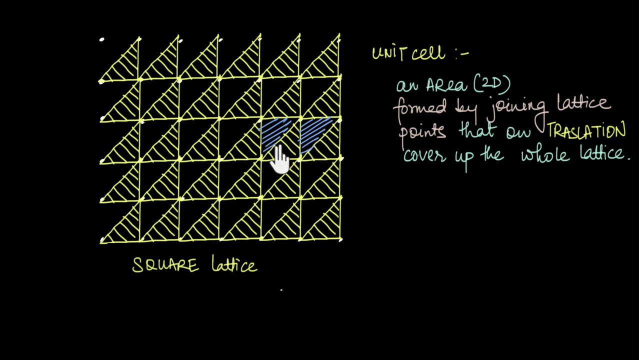 Well, if we took this triangle and if we translated it, if we did that, we will realize that there will always be these gaps that are left behind, right? So a triangle on translation does not cover up a whole two-dimensional space. There will always be these gaps left behind. 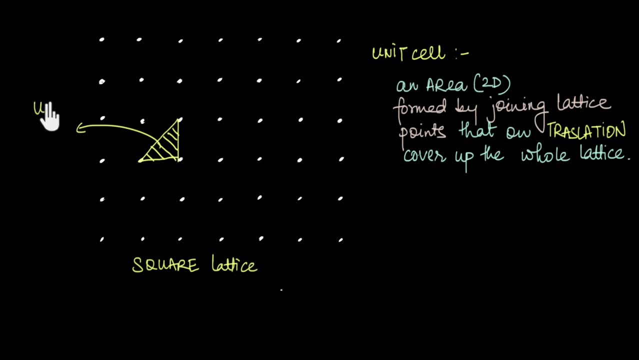 So a triangle cannot be considered to be a unit cell. Now that a triangle is out of the picture, what about using this parallelogram as a unit cell? Well, of course we can use it right If we take this parallelogram and if we translate it. 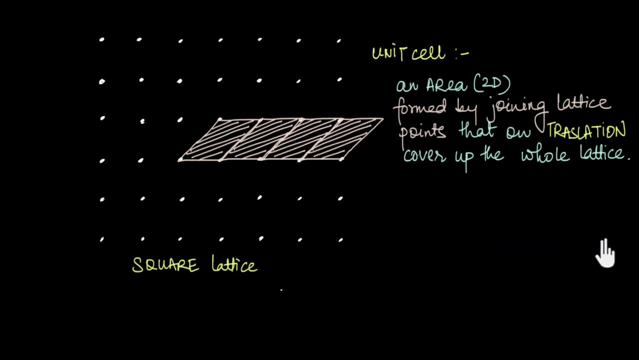 we can see that this parallelogram can cover up the entire space of the lattice, right? So even this parallelogram can be considered as the unit cell Now, because this lattice can now be thought to be made up of these oblique-shaped parallelograms. 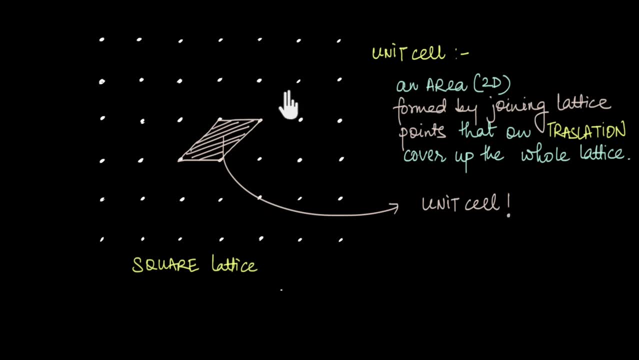 so instead of calling it a square lattice, we might have called it a unit cell. Now if we take this parallelogram and if we translate it, we can see that this parallelogram can cover up the entire space of the lattice, right. 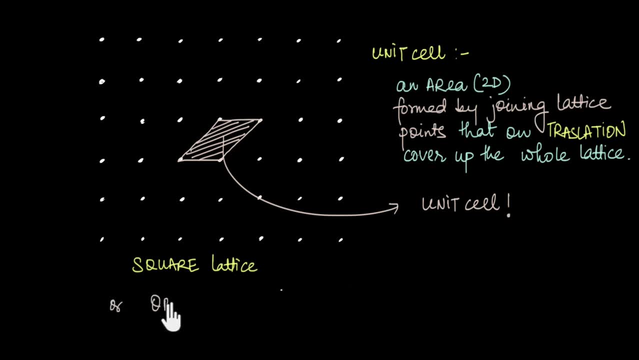 We might have called it an oblique lattice instead. right Now, besides this parallelogram and the square, there are also many other ways of selecting a unit cell. We can, for example, take this rectangle made by joining all these lattice points. 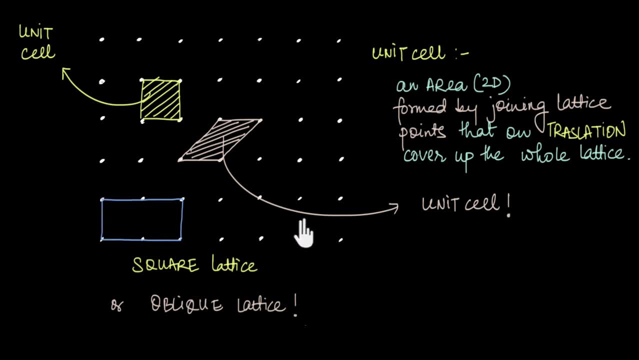 We can think of this as the unit cell, because clearly this rectangle on translation can cover up the whole lattice. Or we might have simply chosen a bigger square, or maybe a longer parallelogram. The choices are actually pretty limitless, because all these shapes on translation can cover up this infinite lattice. 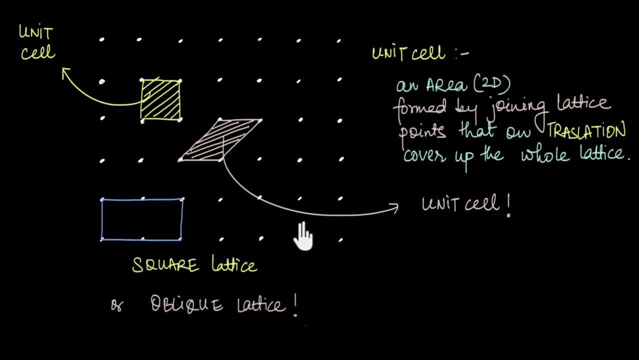 We can think of this as the unit cell, because clearly this rectangle on translation can cover up the whole lattice. Or we might have simply chosen a bigger square, or maybe a longer parallelogram. The choices are actually pretty limitless, Because all these shapes on translation can cover up this infinite lattice. 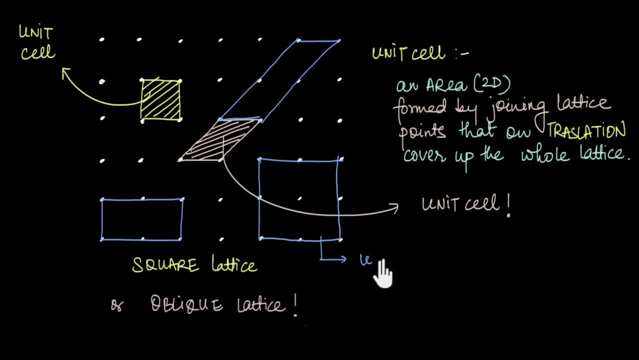 So even all of this can be thought of as the unit cell. However, unlike the square and the oblique, which has lattice points only at the corners, all these other unit cells have lattice points at the corners, but also at some additional places right. 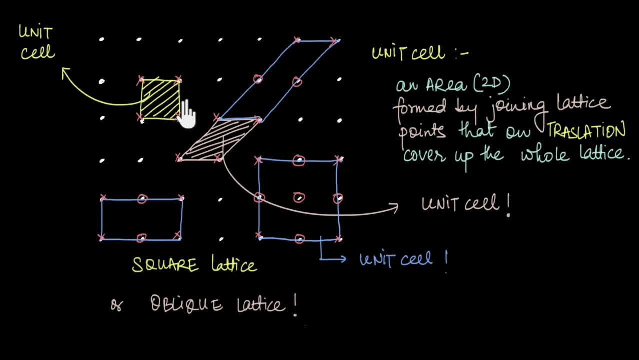 Now, all such unit cells that have lattice points only at the corners, all such unit cells are called the primitive unit cells, While all others, which have lattice points at some other positions also besides the ones at the corners, all such unit cells are not primitive. 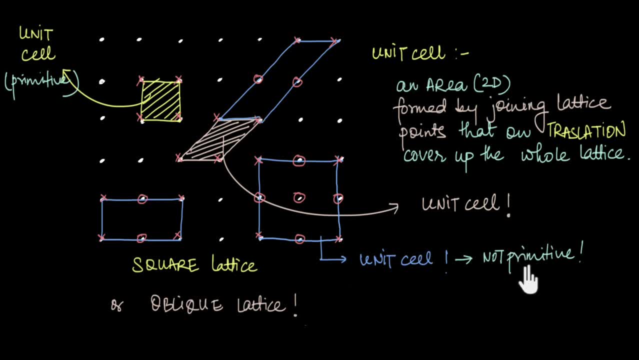 Now, because there can be many different non-primitive unit cells, so therefore we do not focus much on them And instead we generally use these primitive unit cells to describe our overall structure. However, the non-primitive unit cells do play a role sometimes. 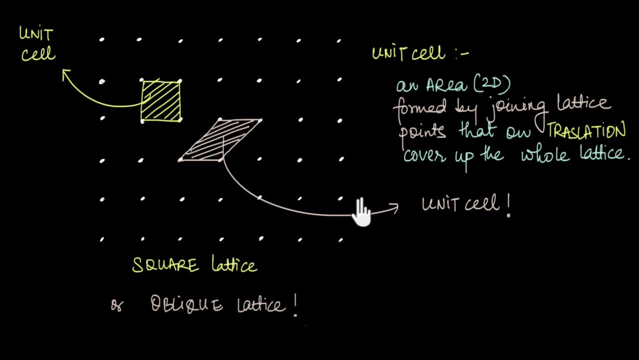 and we'll talk more about this in a future video. Now can you think of some other primitive unit cells that can describe this lattice? Well, actually there are a few more. right, We can think of this lattice to be made up of this kind of oblique unit cells. 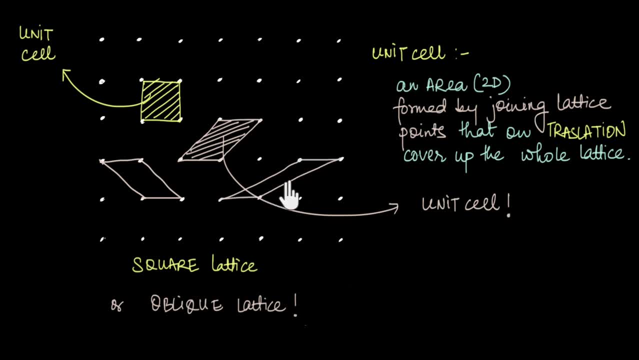 or maybe even these ones which are, like, more oblique. So there are many such ways, but we will go ahead and bunch all of them, We will put all of these together and call them obliques, So because this particular lattice can either be thought to be made up of squares or obliques. 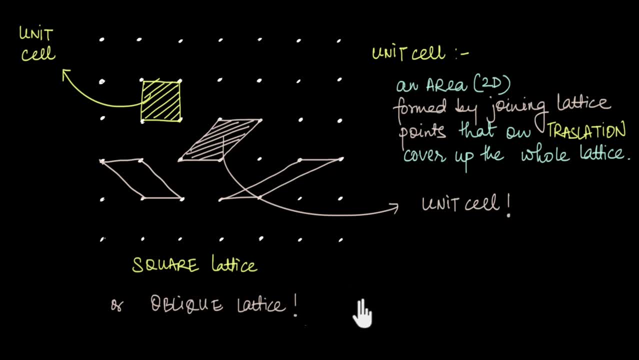 so we should either call it a square lattice or an oblique lattice. But what do we call it? Do we call it square or do we call it oblique? We have to make a decision right, And this decision actually depends upon the unit cell. 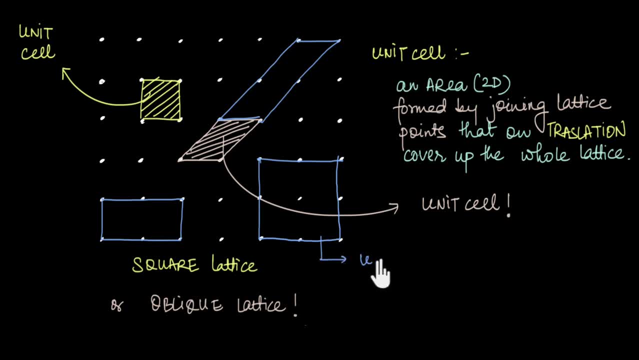 So even all of this can be thought of as the unit cell. However, unlike the square and the oblique, which has lattice points only at the corners, all these other unit cells has lattice point at the corners, but also at some additional places. right now, all such unit cells that 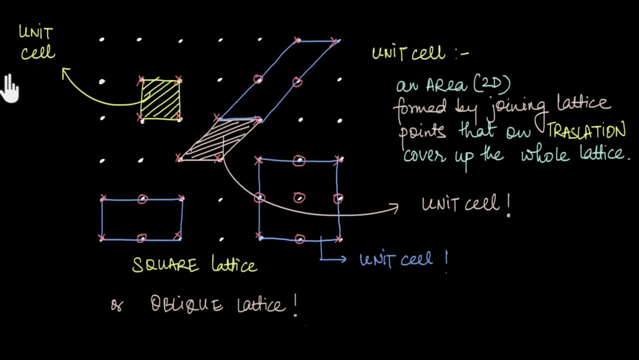 have lattice points only at the corners. all such unit cells are called the primitive unit cells, while all others, which have lattice points at some other positions also besides the ones at the corners, all such unit cells are not primitive. now, because there can be many different non primitive unit cells, so therefore we do not focus much on them and 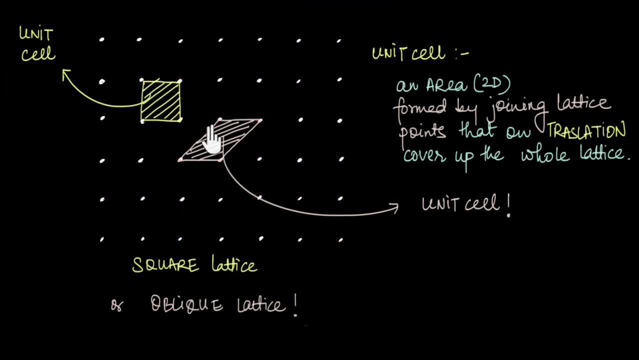 instead, we generally use this primitive unit cells to describe our overall lattice. however, the non primitive unit cells do play a role sometimes, and we'll talk more about this in a future video. now, can you think of some other primitive unit cells that can describe this lattice well? actually, there are a few more, right, we can. 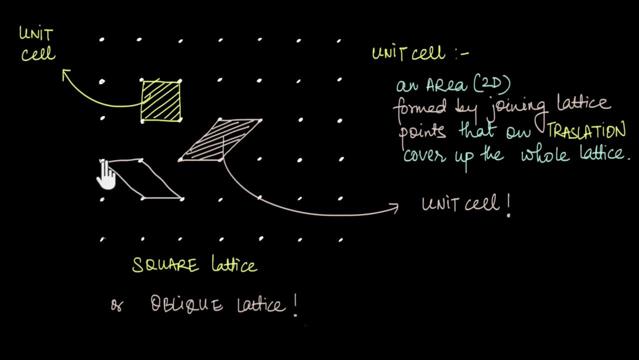 think of this lattice to be made up of this kind of oblique unit cells, or maybe even these ones which are, like, more oblique. so there are many such ways, but we will go ahead and bunch all of these together and call them obliques. so because this particular lattice can either be: 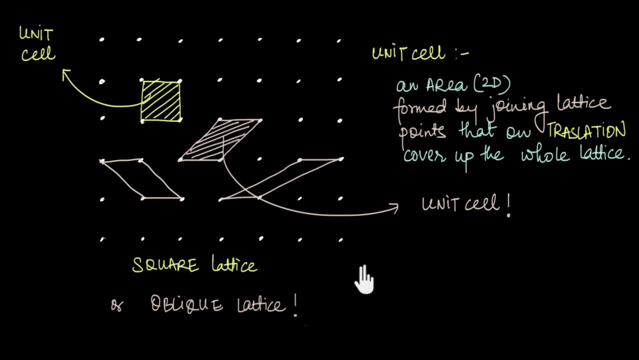 thought to be made up of squares or obliques, so we should either call it a square lattice or an oblique lattice. but what do we call it? do we call it square or do we call it oblique? we have to make a decision right, and this decision actually depends upon the unit cell that best describes. 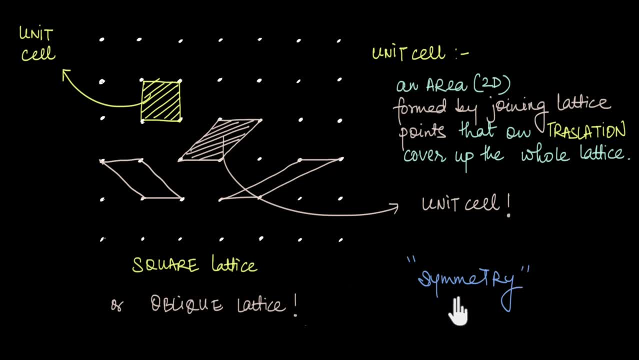 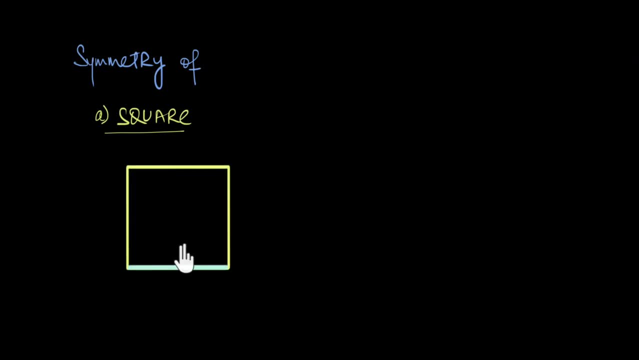 the symmetry of the overall lattice. so what do we mean by this? let's try and understand. so what exactly is a square? well, besides the fact that in a square all the sides are equal and all angles are 90 degrees, if I take a square and try to rotate it along this particular axis, 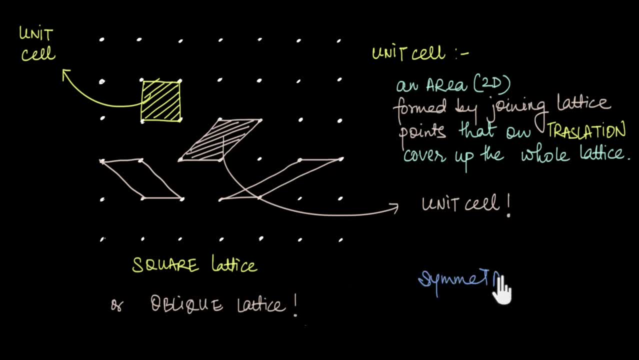 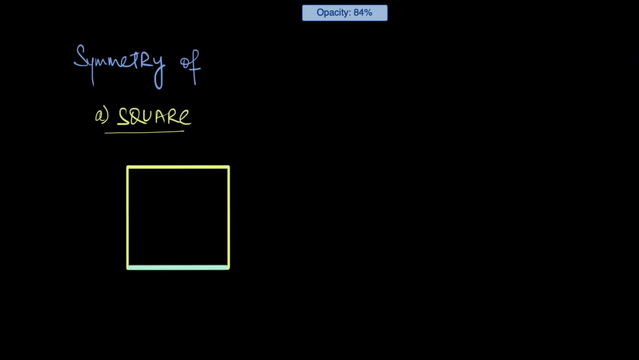 that best describes the symmetry of the overall lattice. So what do we mean by this? Let's try and understand. So what exactly is a square? Well, besides the fact that in a square all the sides are equal and all angles are 90 degrees, 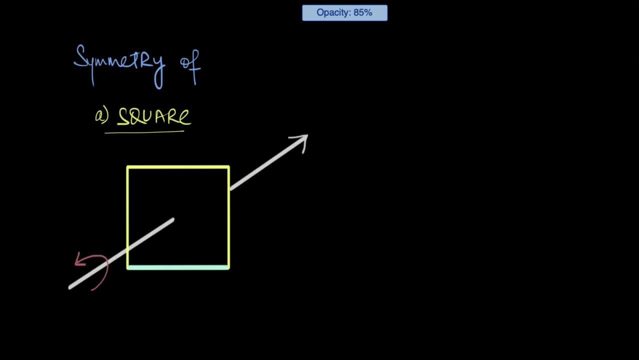 if I take a square and try to rotate it along this particular axis. if I do that, we will see that the square repeats itself after 90 degrees. right, In other words, if I start from my original position and if I rotate this square along this axis by 360 degrees. 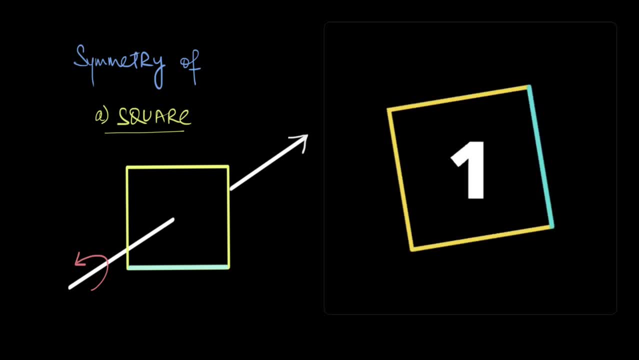 then the square will repeat itself 1,, 2,, 3, and 4 times, right? So we say that this axis has an order 4 and we call it a C4 axis of symmetry. Now, a square also has other axes of symmetry, like this one. 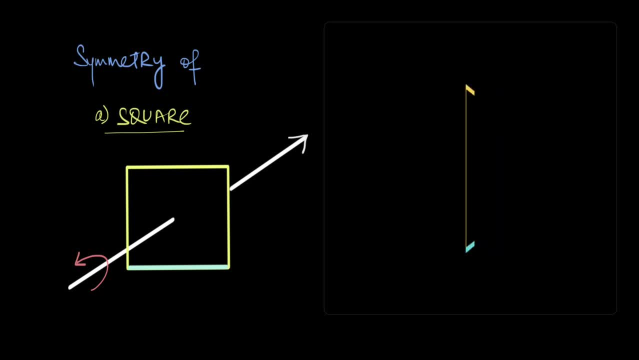 And if we rotate the square by 360 degrees along this axis, the square will repeat itself 2 times. So we call this axis as C2 axis of symmetry. So a square has C4 and C2 axis of symmetry. What about an oblique? 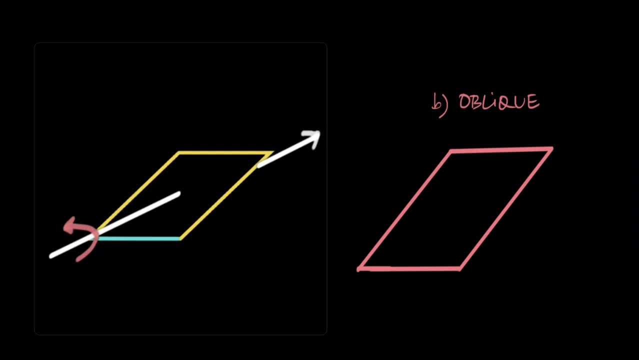 Well, if I rotate the oblique by 360 degrees along this particular axis, then the oblique does not repeat itself after 90 degrees. In fact, it repeats itself only after 180 degrees. And so during a full 360 degree rotation around this particular axis, 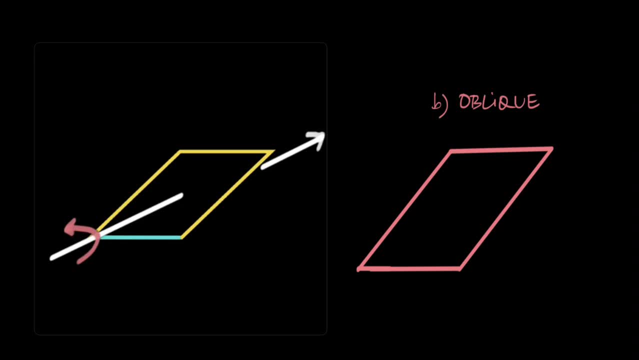 it repeats itself only 2 times. So in an oblique this axis is not a C4 axis, but instead it's a C2 axis of symmetry. Now, if we try rotating the oblique around this axis, then we will see that the oblique repeats itself only after 360 degrees. 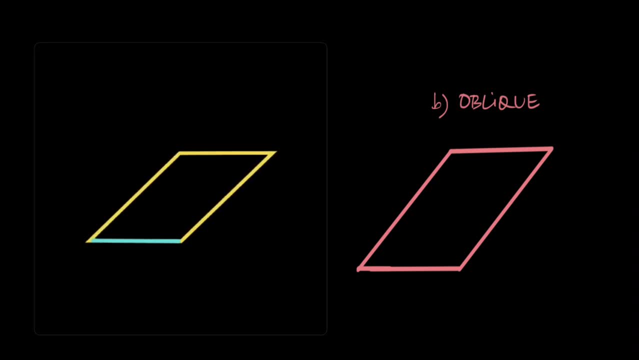 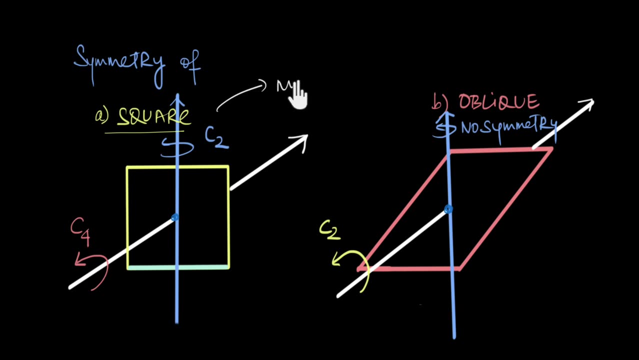 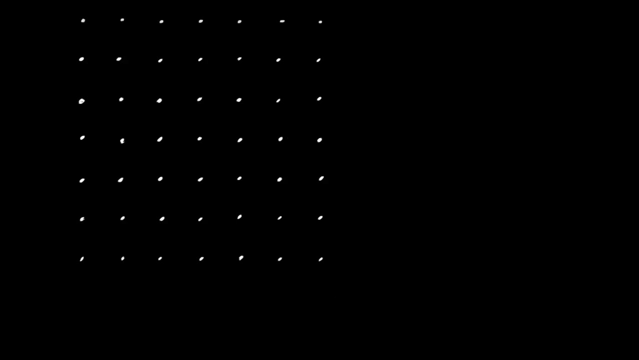 Now, even an asymmetrical object repeats after 360 degrees. right, So this is not a C4 axis, This is not an axis of symmetry. So clearly, a square is much more symmetrical compared to an oblique. right Now, if we come back to our original lattice. 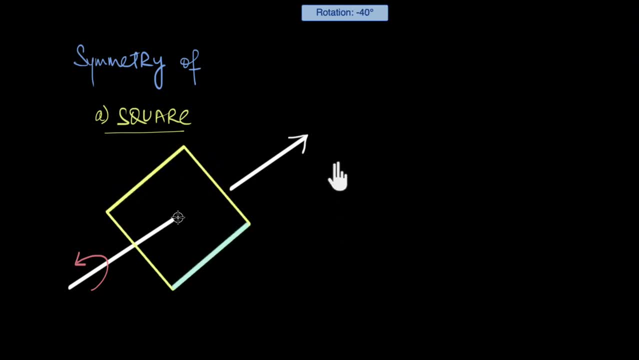 if I do that, we will see that the square repeats itself after 90 degrees, right? in other words, if I start from my original position and if I rotate this square along this axis by 360 degrees, then the square will repeat itself one, two, three and four times, right? so we say that this? 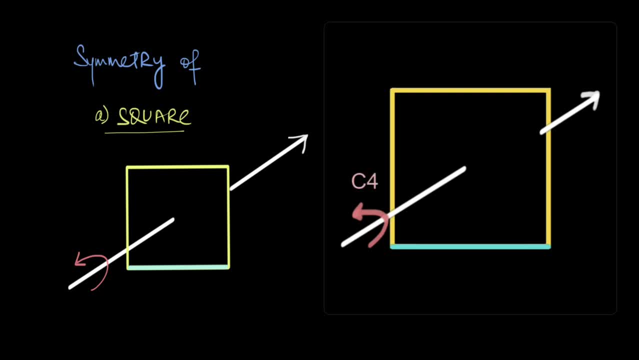 axis has an order four and we call it a C4 axis of symmetry. now, a square also has other axes of symmetry like this one, and if we rotate the square by 360 degrees along this axis, the square will repeat itself times. So we call this axis as C2 axis of symmetry. So a square has C4 and C2. 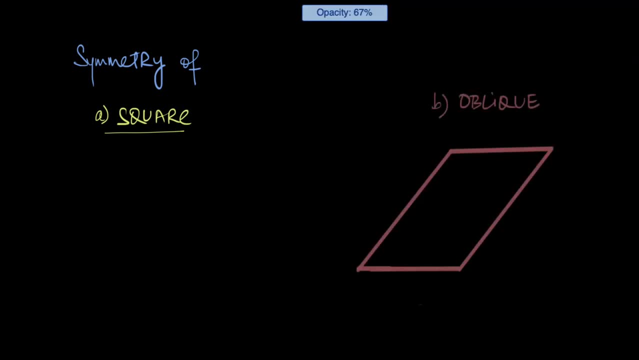 axis of symmetry. What about an oblique? Well, if I rotate the oblique by 360 degrees along this particular axis, then the oblique does not repeat itself after 90 degrees. In fact, it repeats itself only after 180 degrees. and so, during a 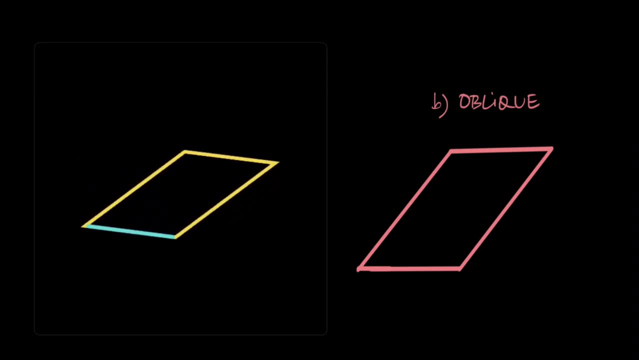 full 360 degree rotation around this particular axis. it repeats itself only two times. So in an oblique this axis is not a C4 axis, but instead it's a C2 axis of symmetry. Now, if we try rotating the oblique around this axis, then we 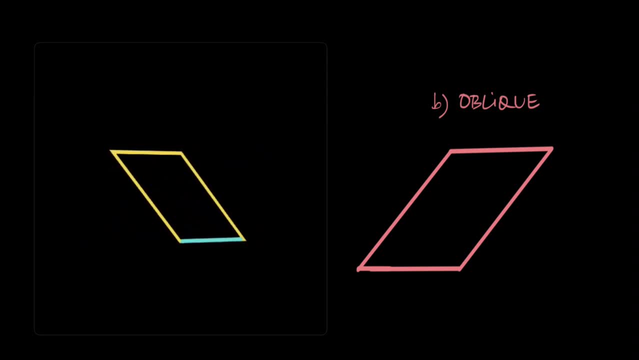 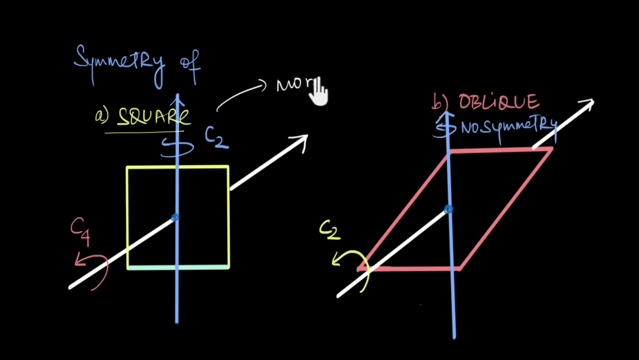 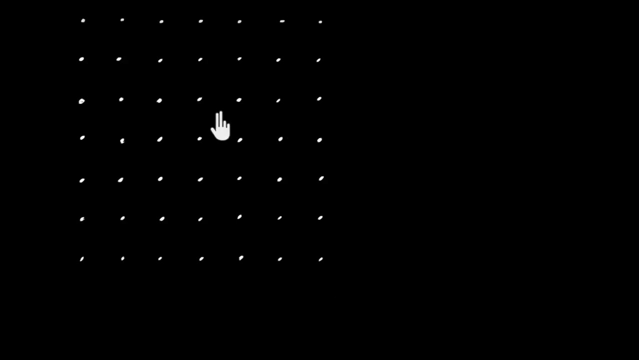 will see that the oblique repeats itself only after 360 degrees. now, even an asymmetrical object repeats after 360 degree, right? so this is not an axis of symmetry. so clearly a square is much more symmetrical compared to an oblique. right now, if we come back to our original lattice and if we try to rotate it- and do remember that these 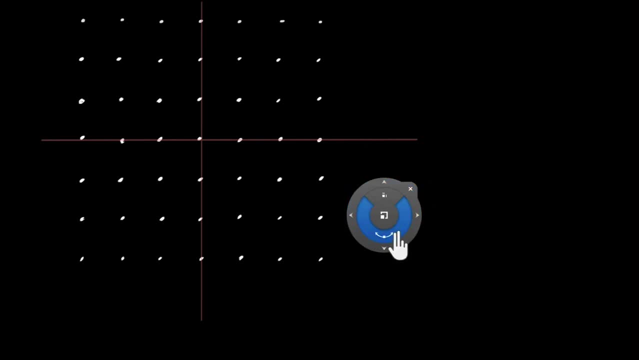 lattices are infinite in all directions, so if i rotate it, the lattice will repeat itself after 90 degrees right, in other words, we can say that this particular lattice has a c4 axis of symmetry, and because a square possesses this symmetry while a parallelogram does not, so a square 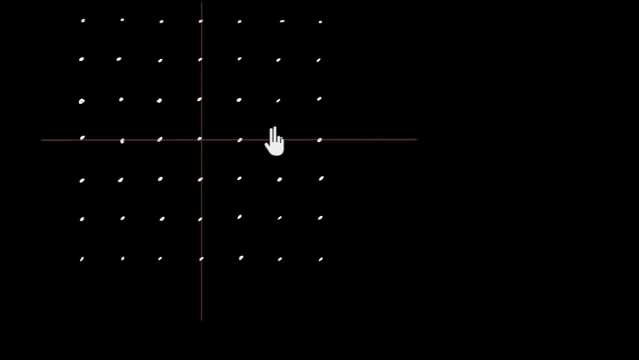 and if we try to rotate it- and do remember that these lattices are infinite in all directions. So if I rotate it, the lattice will repeat itself after 90 degrees right. So if I rotate it, the lattice will repeat itself after 90 degrees right. 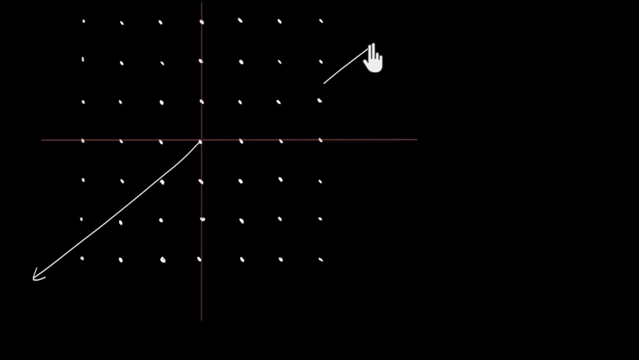 So if I rotate it, the lattice will repeat itself after 90 degrees, right? In other words, we can say that this particular lattice has a C4 axis of symmetry, And because a square possesses this symmetry while a parallelogram does not, 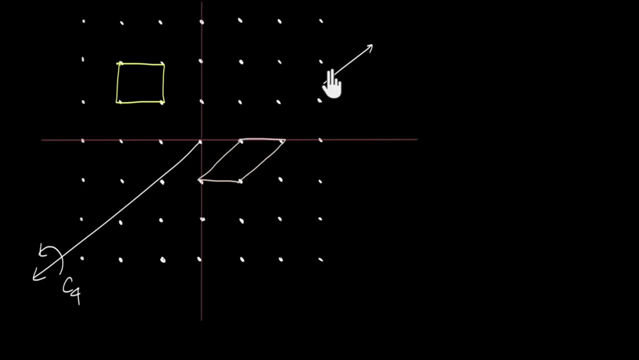 so a square better reflects the global symmetry of the lattice, So we will call this a square lattice. Well, what about this particular lattice? Even this lattice can have both a square as well as a parallelogram as its unit. lattice right. 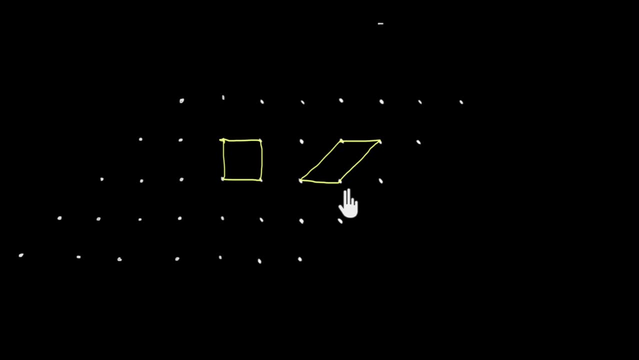 So would you call this a square lattice or would you call this an oblique lattice? Well, if I took this particular lattice and tried rotating it- and do remember that this lattice is actually infinite in all directions- So if I try rotating this lattice, 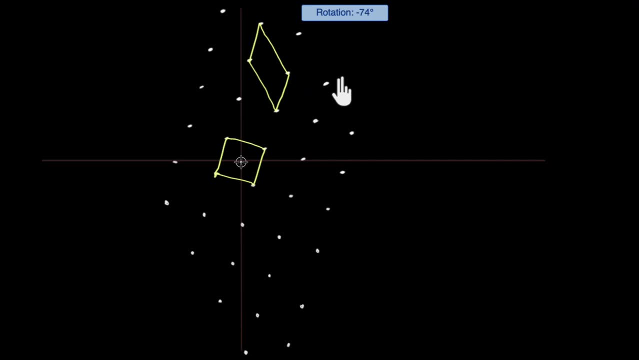 the lattice will actually repeat itself after 90 degrees, right? So you can see that this square has repeated itself after 90 degrees, right? So you can see that this square has repeated itself after 90 degrees, right? While the oblique has not repeated itself. 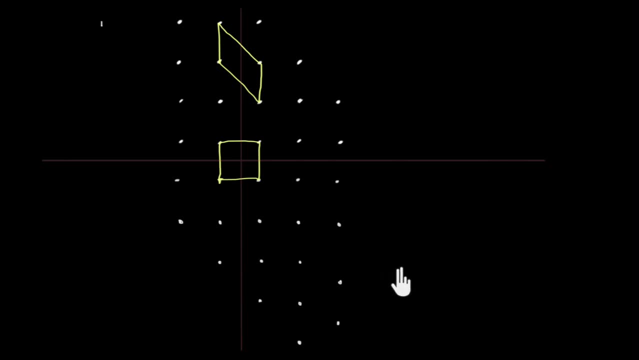 So because this lattice is infinite in all directions, the global symmetry of the lattice is better described by this square rather than this oblique. So even out here we will call this a square lattice. So we can now conclude and say that if there is more than one unit cell that can describe the overall lattice, 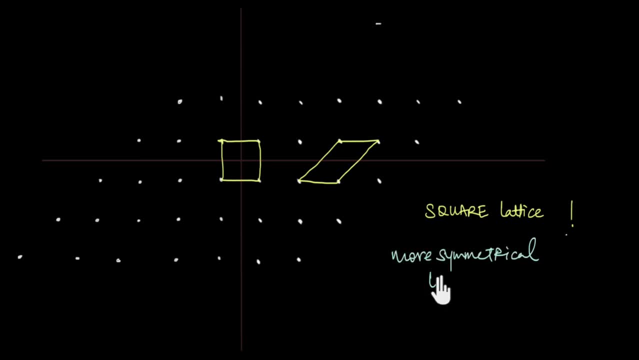 we should actually choose the more symmetrical lattice, more symmetrical unit cell, as the more symmetrical unit cell will better describe the global symmetry of the lattice. So now that we have understood what a unit cell is and which unit cell should be chosen to describe a particular lattice, in the next video we are going to talk about 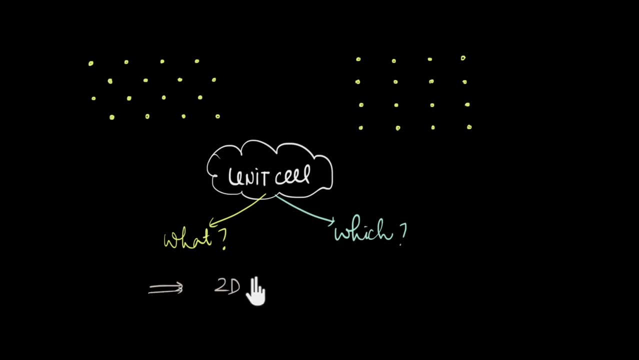 different Bravais lattices in two dimension and three dimension, and we are going to classify them into different categories. So see you in the next video.